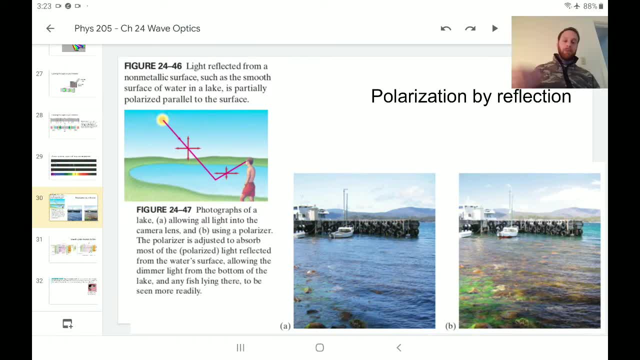 than it is to shake within the surface. So after light reflects off of water, for example, it is more polarized left-right than it is up and down, And it is this reason why it's important, especially if you're a fisherman- you know fishing, I guess near dusk or not quite at dusk, but around sunset or later in the day- you want to have polarizers, polarized sunglasses rather, that are oriented in such a way to block out that left-right polarization. In other words, you 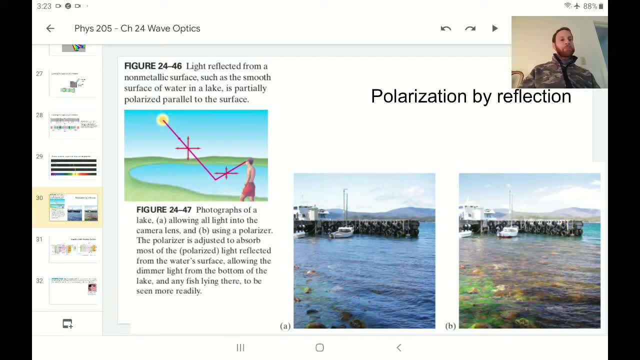 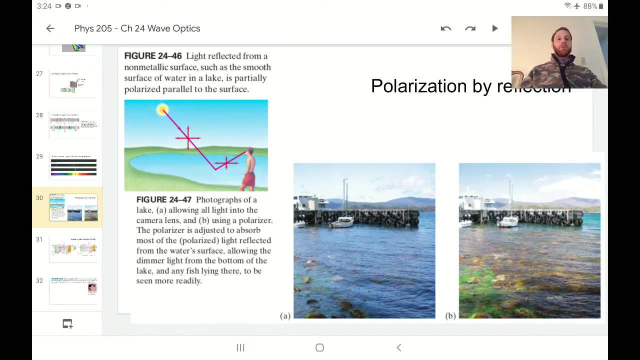 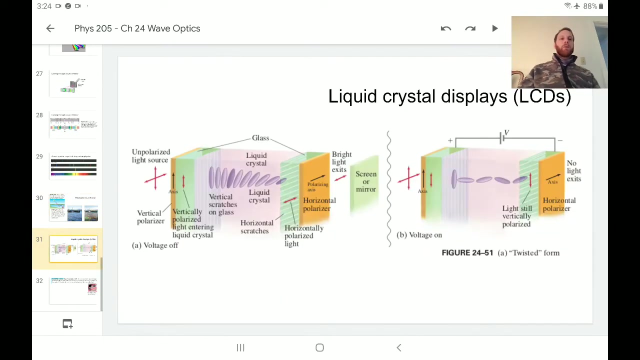 you'd like your sunglasses to be polarized vertically, And likewise. this other example here has to do with: well, if you take a picture of you know some water without a polarizer- and with a polarizer you know- you can see the difference in being able to filter out that extra reflection that you get from the surface. Liquid crystals displays, as advertised, involve. it seems a bit busy here, but I claim it's not. 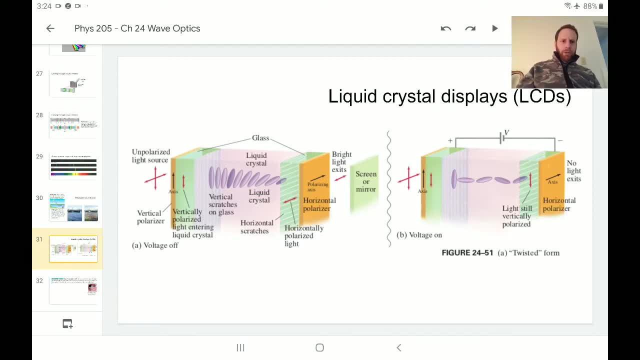 too complicated Liquid crystals. you can think of them in the same way as a kind of polarizing material. So at least the basic structure of the liquid crystal display has a- you know- polarizer on two ends. Light can come through And as the liquid crystal, it interacts. each liquid crystal interacts with another one in a way that they kind of want to line up together, if they can. They're permanently oriented to be. 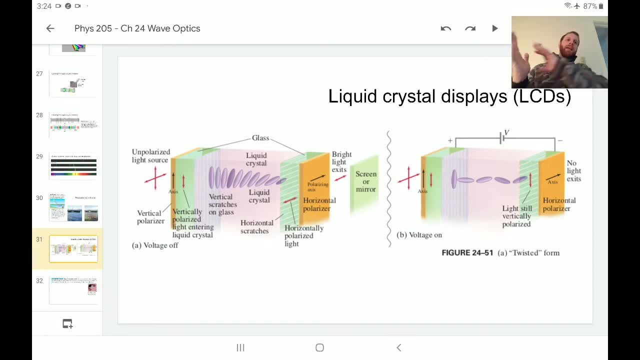 let's say vertical and horizontal on these two separate surfaces, But throughout that fluid. it's a fluid with these long, sort of long, rigid, rod-like molecules. They'll sort of slowly try to go from one orientation to another And that can make some incoming- which is now linearly polarized light, let's say up and down, slowly rotate throughout the material and come out the other side. On the other hand, if you do apply a voltage to it, which means applying an electric field, you can mess up that nice pattern of liquid crystals. 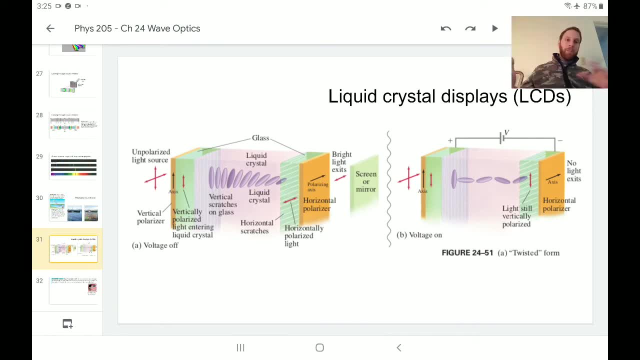 where they're lining up with each other And that basically stops this natural- if you want to call it that way- rotation of light inside of that material, which means that linearly polarized vertical coming in can't get rotated, And once it hits that other side or the or the filters oriented the other way, basically no light gets through. And that is the basic, or into a basic setup of liquid crystal display. Okay so, 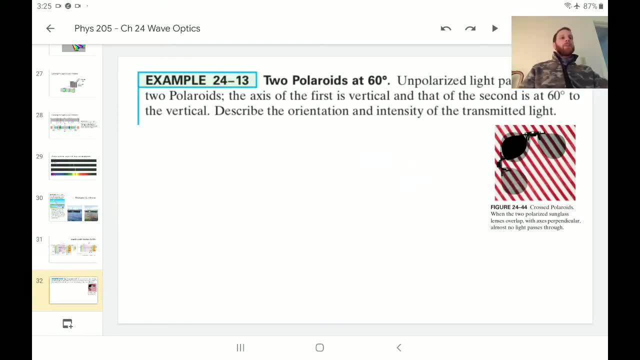 let's do one example. This example has to do with polarizers which, by the way, again, you can imagine just taking some sunglasses and polarized sunglasses and any one of them would act as a polarizer, But two polarizer at 60 degrees. So you know, unpolarized light passes through two polar polarides. the axis of the first is vertical and that of the second is 60 degrees to the vertical describe the orientation and intensity. So let's see if I can just work through this on the screen. 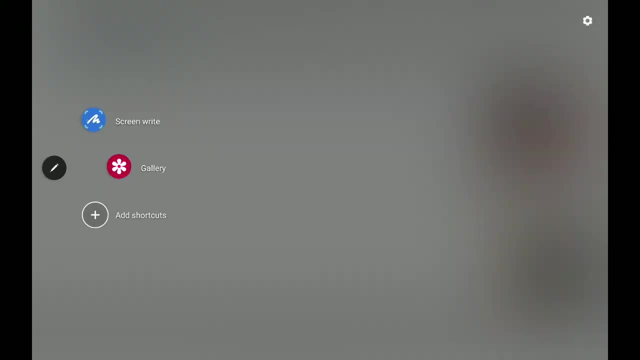 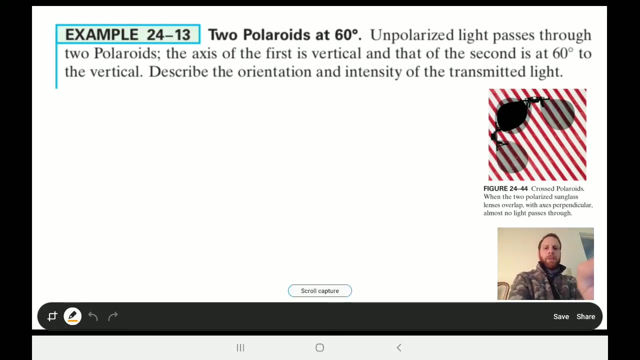 Okay. so I think the basic picture here is that you've got initially unpolarized lights coming through, And so that's vertical, and I'll have this going, let's say, in and out, And then I will draw my two polarizers in green. So the first one is vertical, So that's good, So I'm showing it in green, I'm going to draw my two polarizers in green And then I'm going to draw my 360 degrees. So next thing between this is my блокer And I'm going to draw my three polarizes in green here, And when I'm done with that, I'm going to draw my three raw light. So I'm running some Excel data on this panel here And everything is sent to zero. So it's all realized here. So if you draw this one, I'm going to needle through that line here and then I'm going to use a live color to do this answer. Now, each I would use the zip tag mark and it should be. eyesight is correct for me, And let's go and even stands. 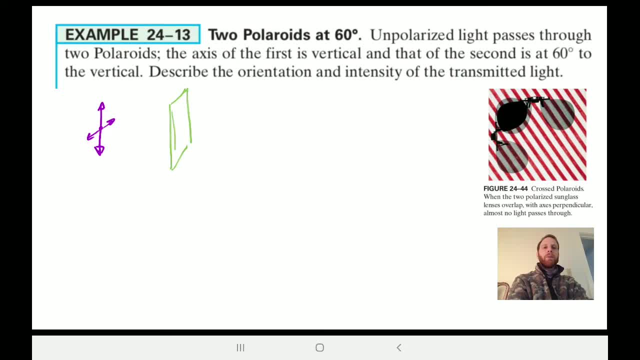 This is going to be like the lecture, And then the second one is 60 degrees with respect to that, So it's somehow oriented and I don't know how crappy this is going to turn out. Yeah, it could be worse. So let's suppose that this has been oriented 60 degrees. 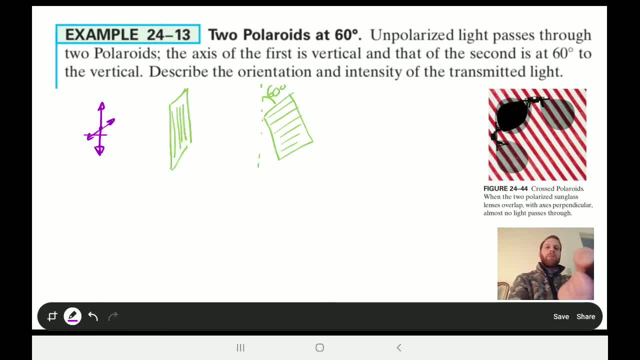 Okay, So good, We can draw some intermediate stuff, That light that comes in. we know that because of the orientation of this polarizer being vertical, that means all the horizontal stuff doesn't get through, but all the vertical stuff does. 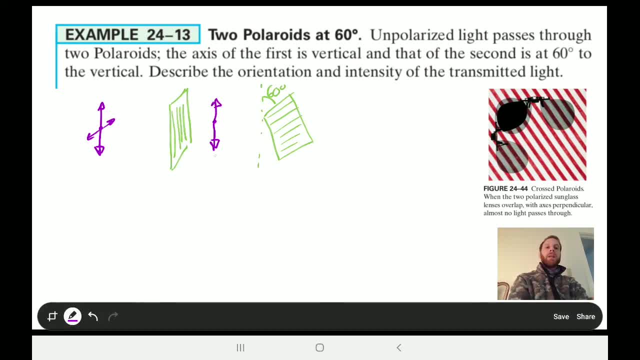 And we had already seen what the intensity here should look like compared to here, If this original intensity is I0, we know that this and let's see, I'm going to call this filter number 1 and I'll call this filter number 2.. 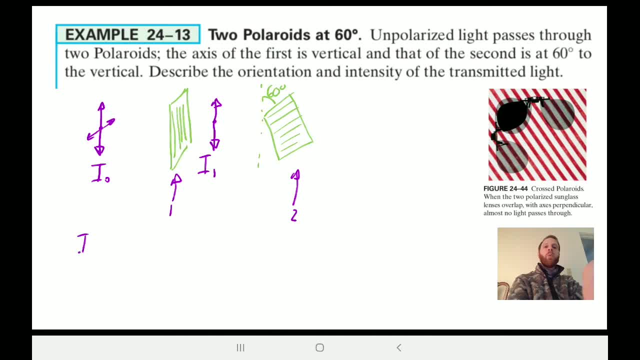 The intensity here I'll call I1.. We know that I1.. I1 is half of the intensity of the original unpolarized light. Okay, cool, Then this polarized light passes through another polarizer and some amount of light will make it through. 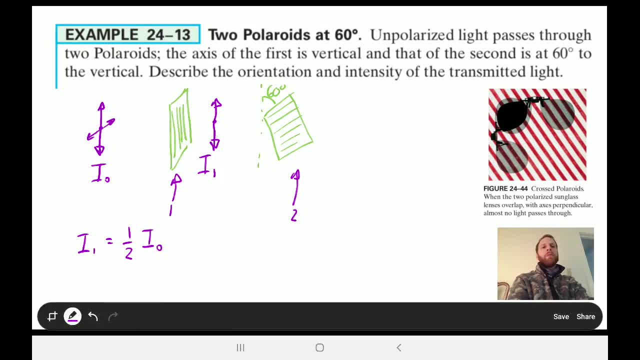 but only the fraction or the component of the initial. you know we're talking about electric field. basically, that can make it through here, And so what we expect to emerge is light that is polarized in the same direction as this axis of this polarizer, so it'll go in that same direction. 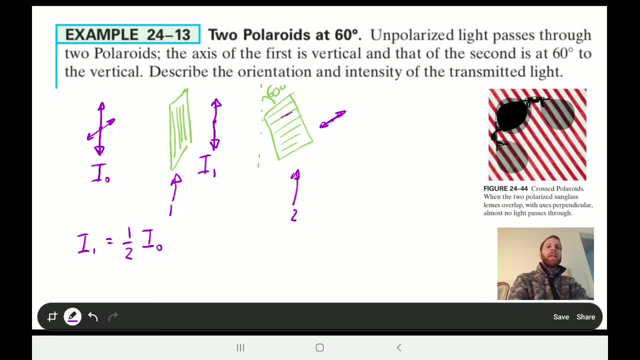 but we do expect that it will be smaller, because we're only getting the component of this, We're only getting the component of that that makes it through, And so remember how this works. is that the intensity after that second polarizer. it's related to the intensity of light that came through before. 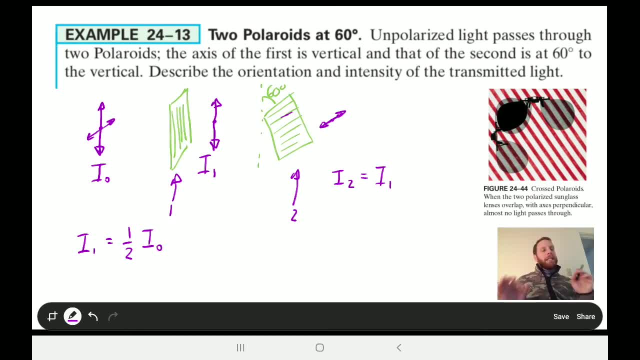 but then involves a cosine of an angle. It's actually the electric field. The electric field involves the cosine, so let me remind you what this would involve. You don't need to do all these details. I'll only remind you where it comes from. 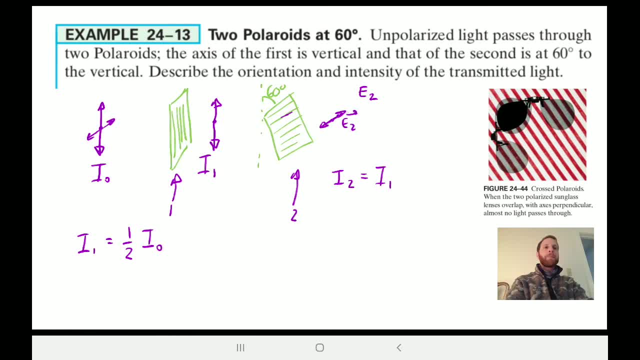 The electric field as it comes out. let's call this E2, and this is E1.. E2 has a magnitude which is related to E1 times the cosine of the angle between, you know, E1 and E2, and really that is the 60 degrees. 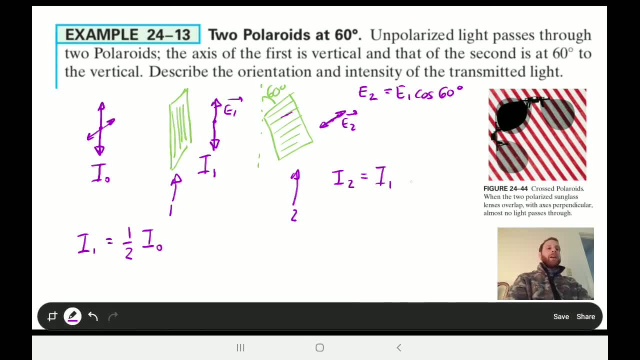 However, the intensity involves the intensity of light. Okay cool, Okay cool. So the cosine of light involves the square of the electric field and therefore it involves the square of the cosine. So perhaps I should, more carefully, just write this as cosine of theta, where this angle is theta. 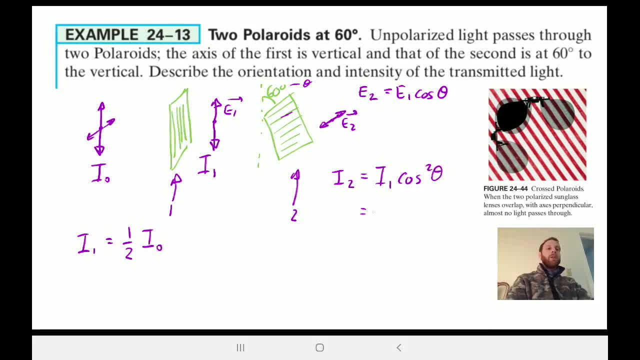 And this is cosine squared of theta. In other words, for us this is the intensity of the first one, which is one-half intensity- not That's what we had found over here- And then this is cosine squared of 60 degrees.